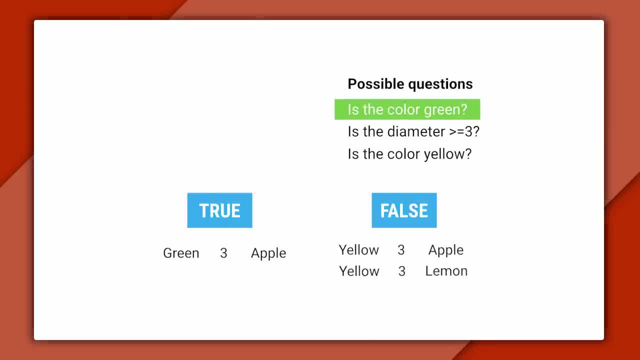 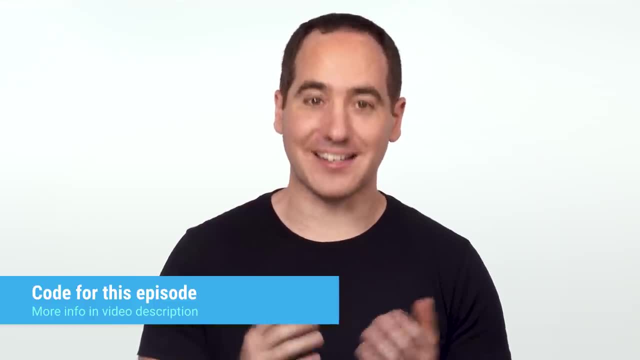 On the way. we'll cover concepts like decision tree learning, Gini, impurity and information gain, And you can find the code for this episode in the description, and it's available in two formats, both as a Jupyter notebook and as a regular Python file. Okay, let's get. 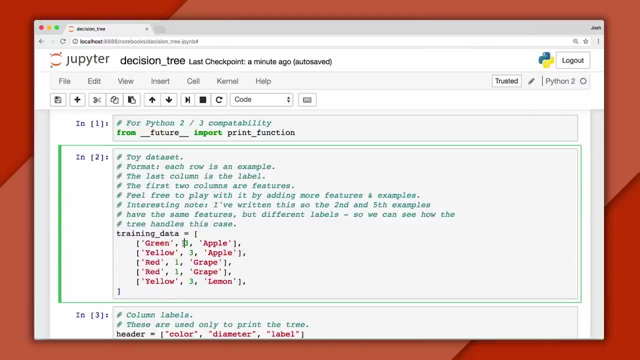 started. For this episode, I've written a toy dataset that includes both numeric and categorical attributes, And here our goal will be to predict the type of fruit, like an apple or a grape, based on features like color and size. At the end of the episode, 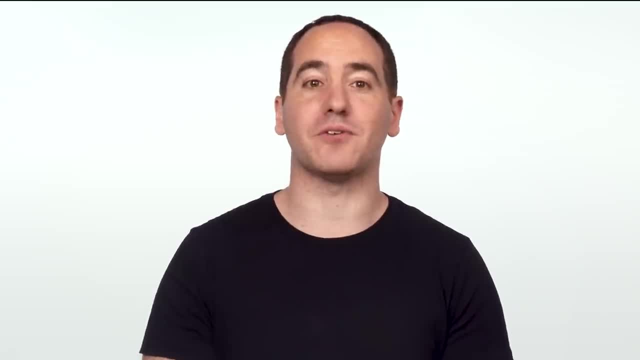 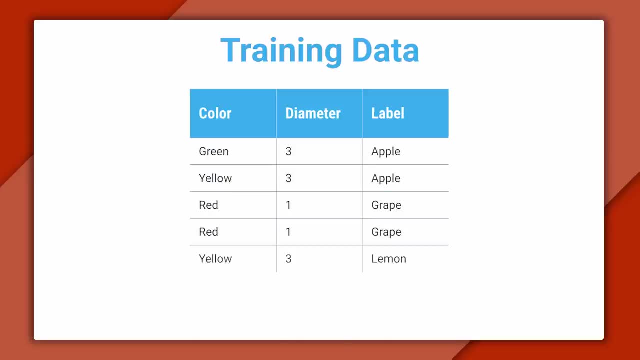 I encourage you to swap out this dataset for one of your own and build a tree for a problem you care about. Let's look at the format. I've redrawn it here for clarity. Each row is an example And the first two columns provide features or attributes that describe the data. The 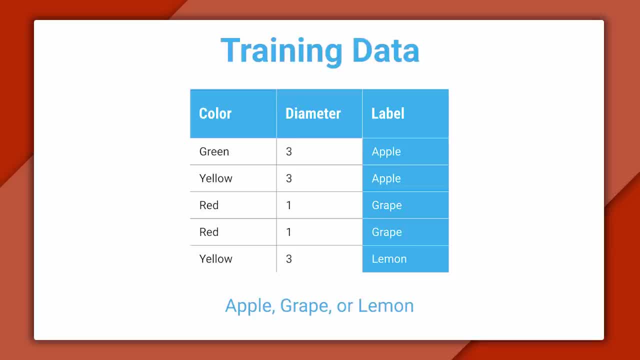 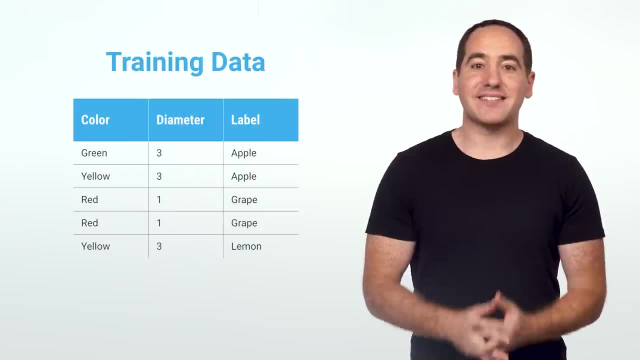 last column gives the label or the class we want to predict And, if you like, you can modify this dataset by adding additional features or more examples, and our program will work in exactly the same way. Now this dataset is pretty straightforward, except for one thing. 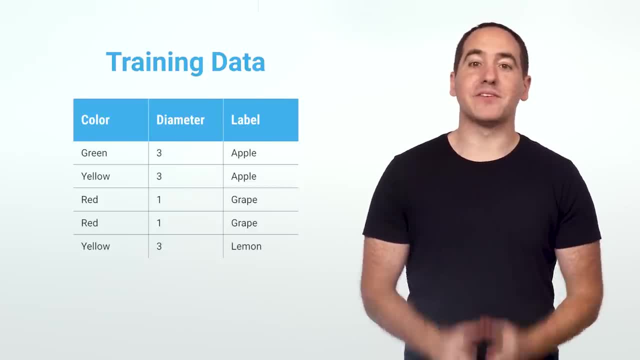 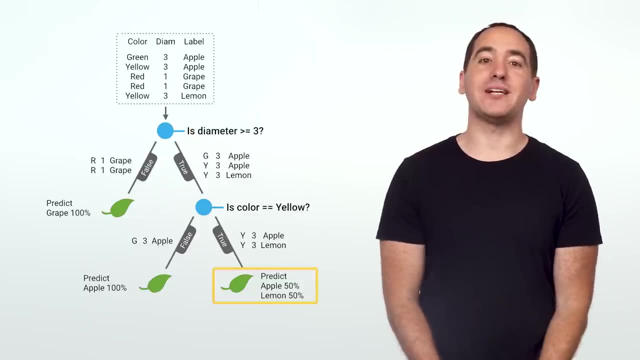 I've written it so it's not perfectly separable, And by that I mean there's no way to tell apart the second and fifth examples. They have the same features but different labels, And this is so we can see how our tree handles this case. 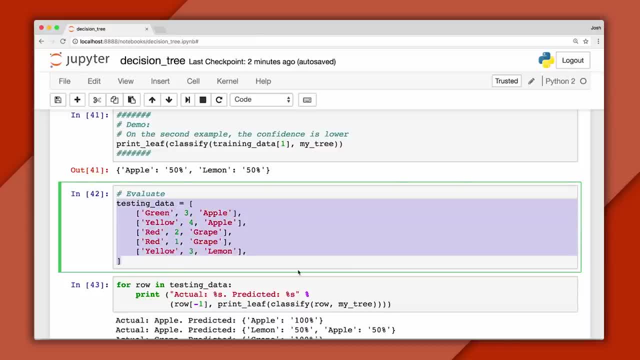 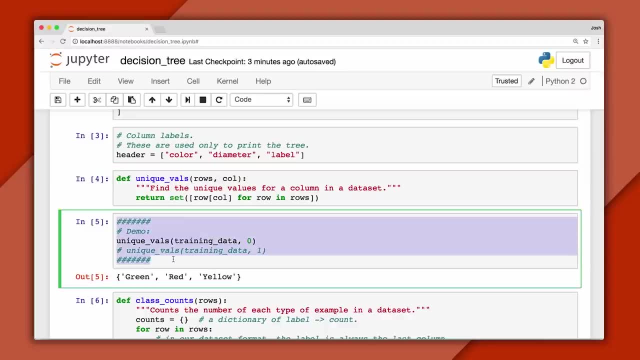 Towards the end of the notebook, you'll find testing data in the same format. Now I've written a few utility functions that make it easier to work with this data, And below each function I've written a small demo to show how it works, And I've repeated 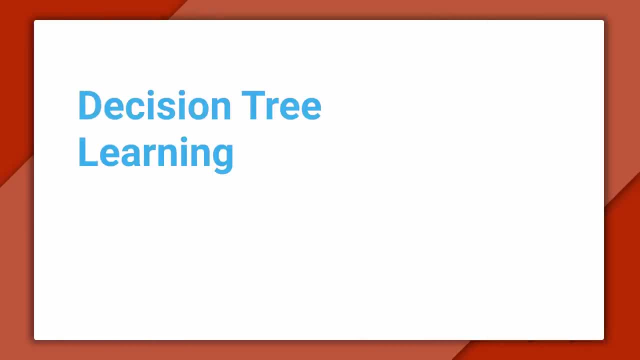 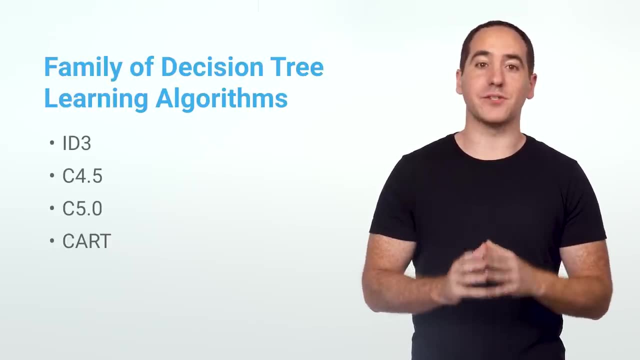 this pattern for every block of code in the notebook. Now, to build the tree, we'll use a decision tree learning algorithm called CART And, as it happens, there's a whole family of algorithms used to build trees from data At their core. 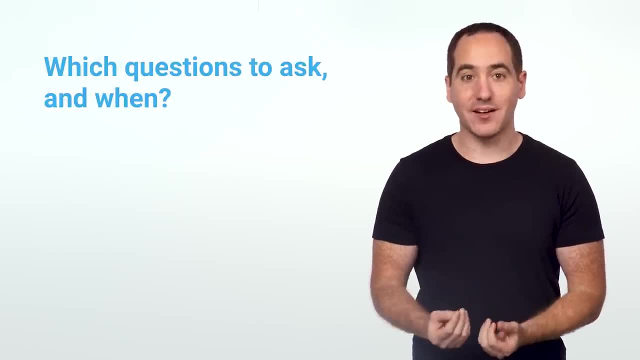 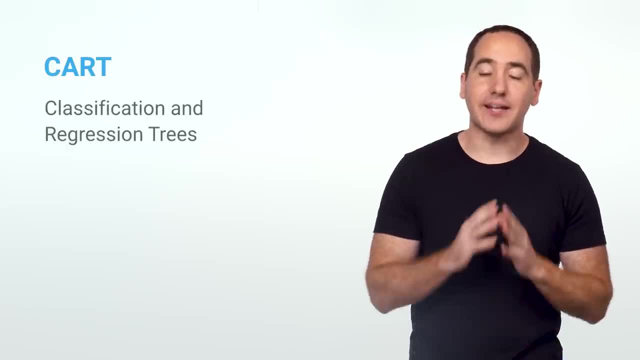 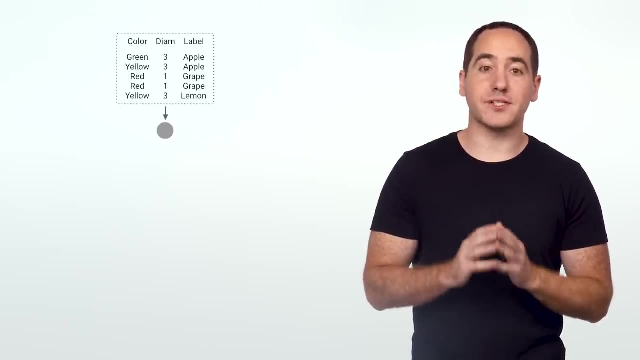 CART stands for Classification and Regression Trees, And here's a preview of how it works. To begin, we'll add a root node for the tree And all nodes receive a list of rows as input, and the root will receive the entire training set. Now each node will ask a true, false. 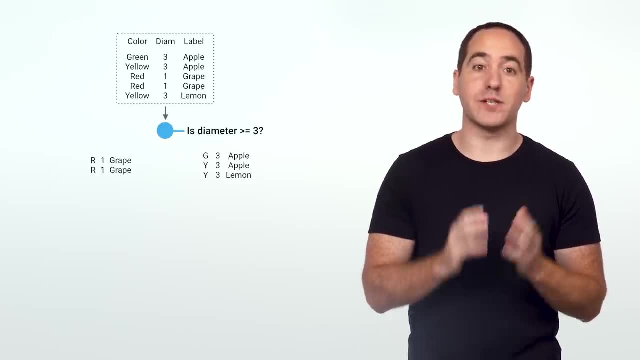 question about one of the features And in response to this question, we split or partition the data into two subsets. These subsets then become the input to two child nodes we add to the tree, And the goal of the question is to… unmix the labels as we proceed down. 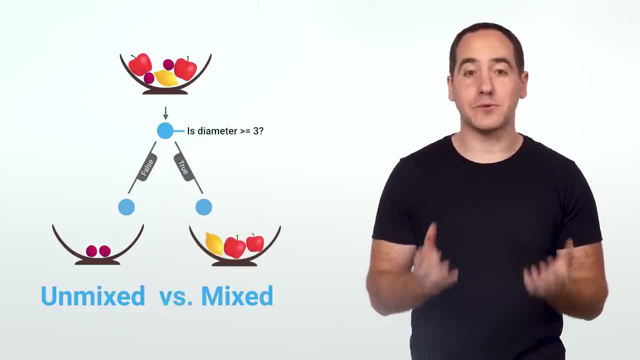 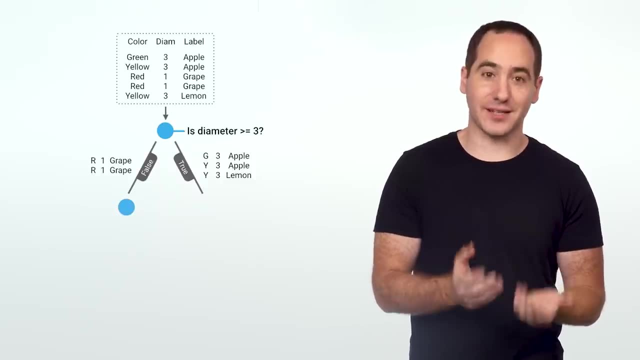 Or in other words, to produce the purest possible distribution of the labels at each node. For example, the input to this node contains only a single type of label, so we'd say it's perfectly unmixed. There's no uncertainty about the type of label. 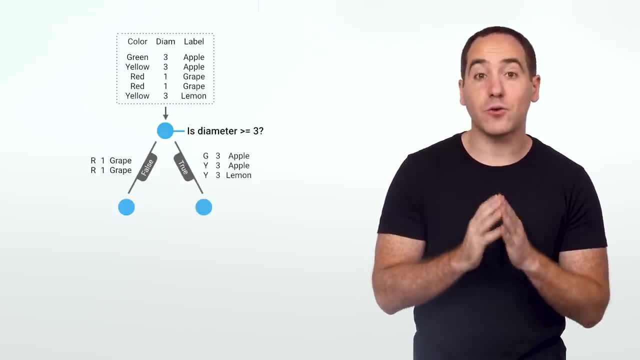 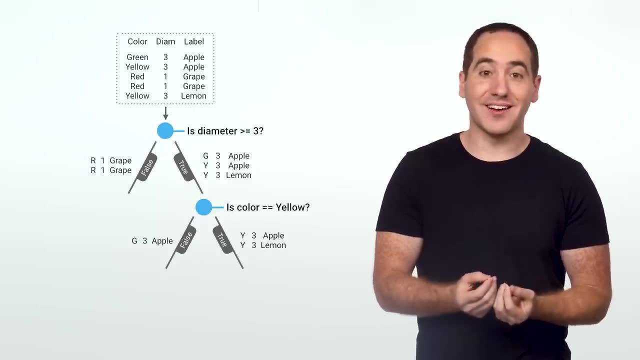 On the other hand, the labels in this node are still mixed up, so we'd ask another question to further narrow it down. And the trick to building an effective tree is to understand which questions to ask and when. And to do that we need to quantify how much a question helps to unmix the labels. 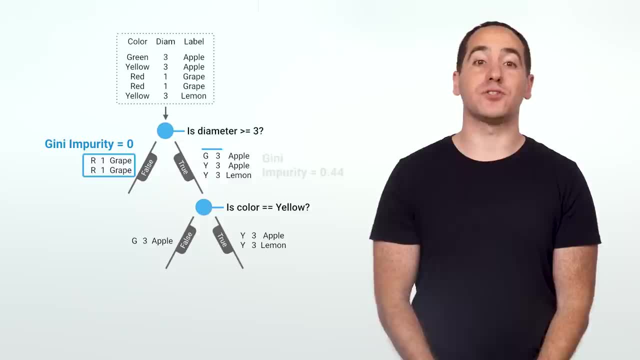 And we can quantify the amount of uncertainty at a single node using a metric called Gini impurity. And we can quantify how much a question reduces that uncertainty using a concept called information gain. We'll use these to select the best question to ask at each point. 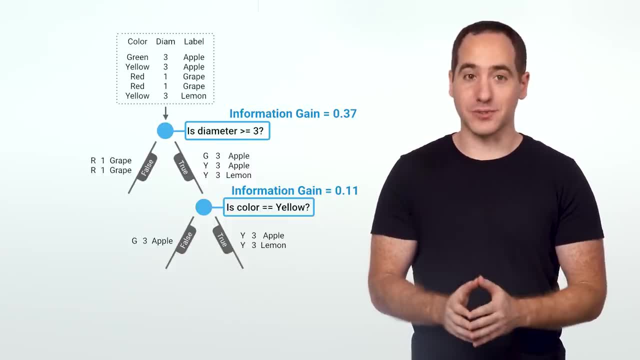 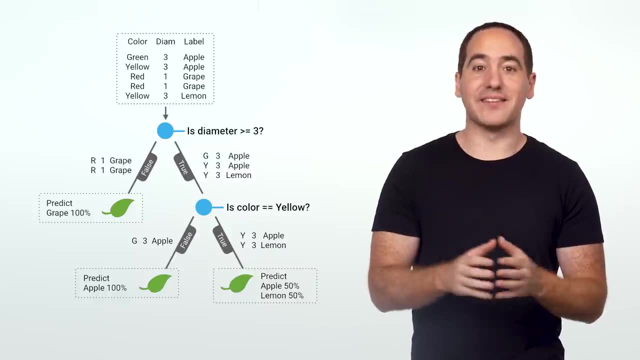 And, given that question, we'll recursively build the tree on each of the new nodes. We'll continue dividing the data until there are no further questions to ask, at which point we'll add a leaf To implement this. first we need to understand what type of questions can we ask about the data. 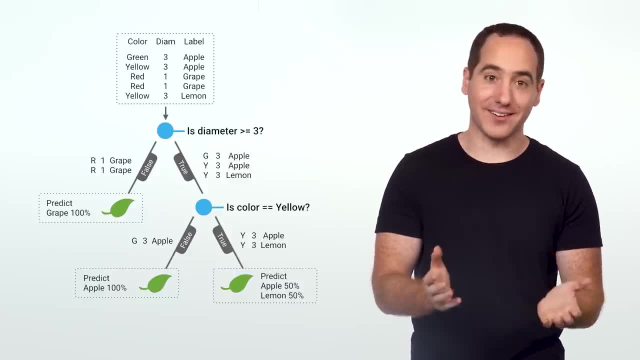 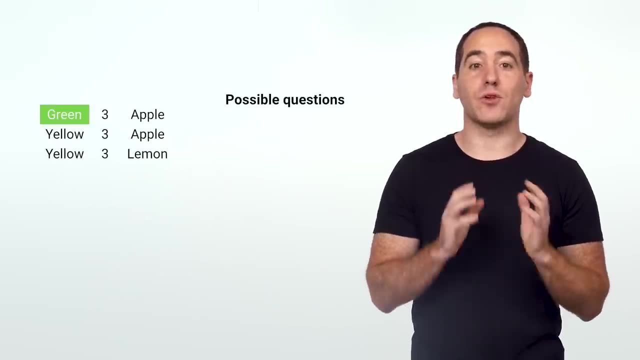 And second, we need to understand how to decide which question to ask. when Now, each node takes a list of rows as input And to generate a list of questions, we'll iterate over every value for every feature that appears in those rows. Each of these becomes a candidate for. 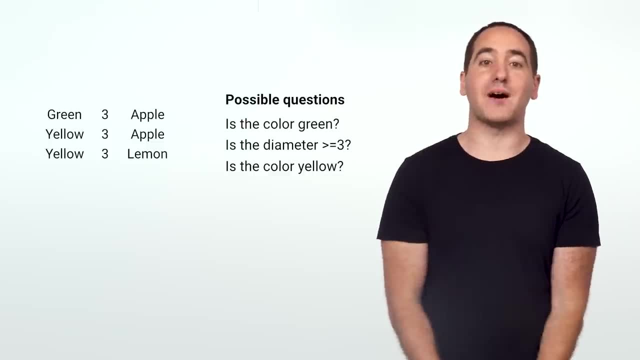 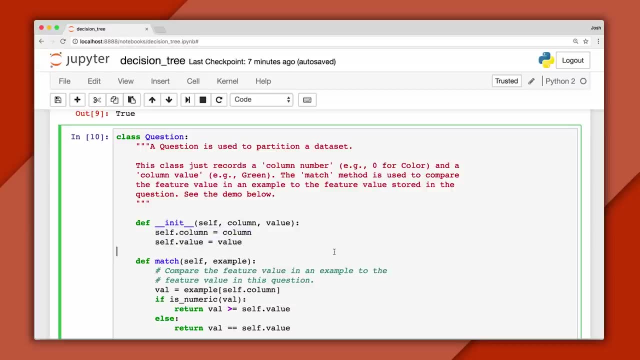 a threshold we can use to partition the data, And there will often be many possibilities. In code. we represent a question by storing a column number and a column value, or the threshold we'll use to partition the data. For example, here's how we'd write a question to test if the color is green. 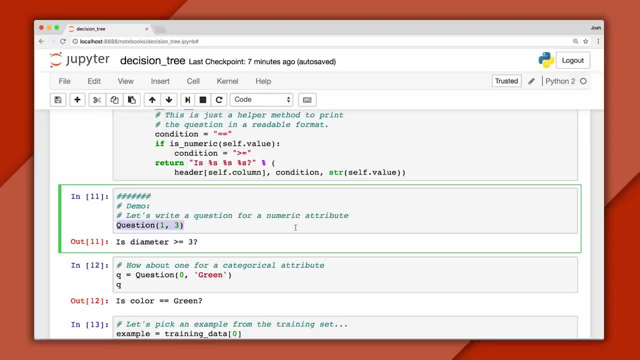 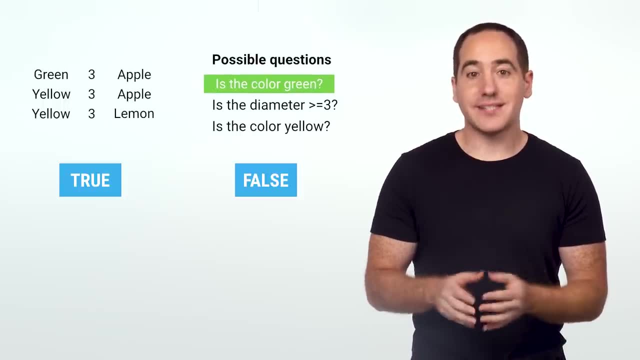 And here's an example for a numeric attribute to test if the diameter is greater than or equal to three. In response to a question, we divide or partition the data into two subsets. The first contains all the rows for which the question is true and the second contains everything else. 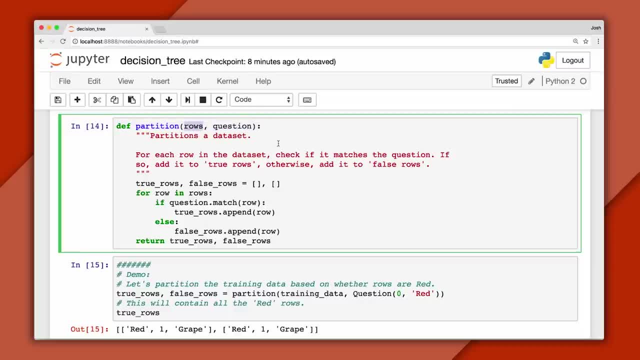 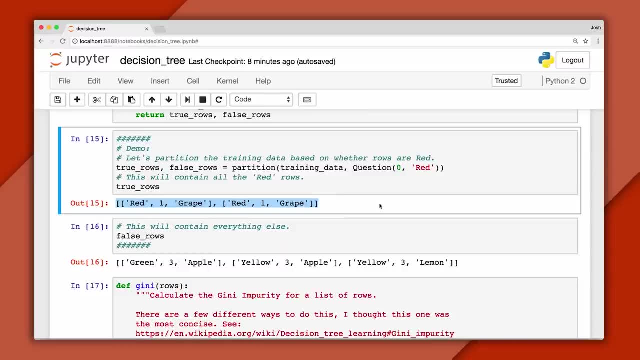 In code. our partition function takes a question and a list of rows as input. For example, here's how we partition the rows based on whether the color is red Here. true rows contains all the red examples and false rows contains everything else. 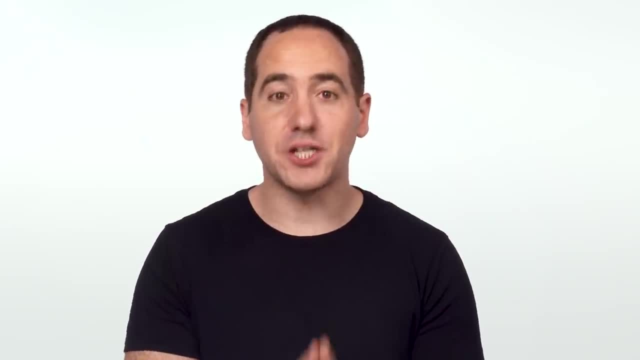 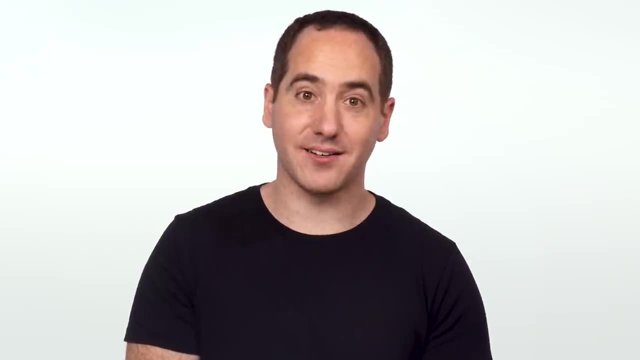 The best question is the one that reduces our uncertainty the most: Ngini impurity lets us quantify how much uncertainty there is at a node. Information gain will: let us quantify how much a question reduces that. Let's work on impurity first. Now, this is a metric that ranges between zero and one. 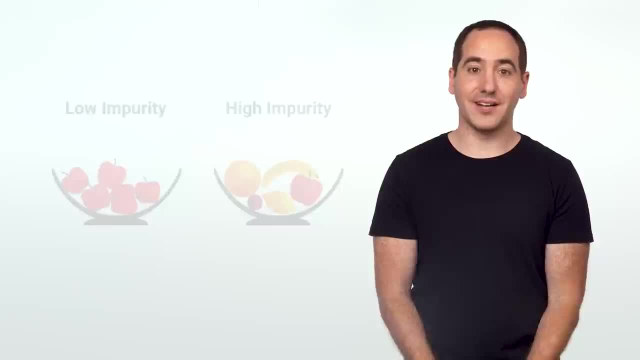 where lower values indicate less uncertainty or mixing at a node. It quantifies our chance of being incorrect and it's a good way to measure our uncertainty. It's a good way to measure our uncertainty. It's a good way to measure our uncertainty. 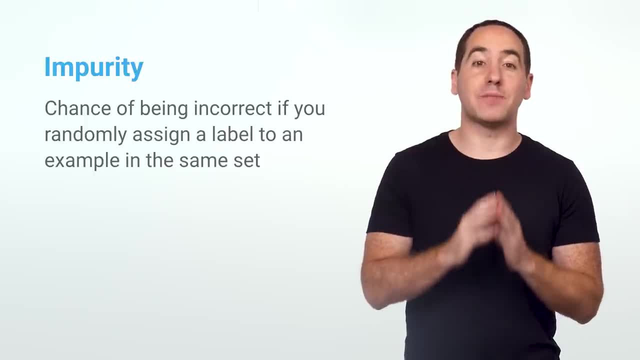 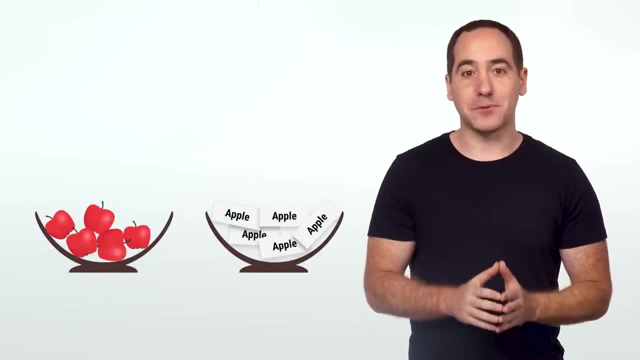 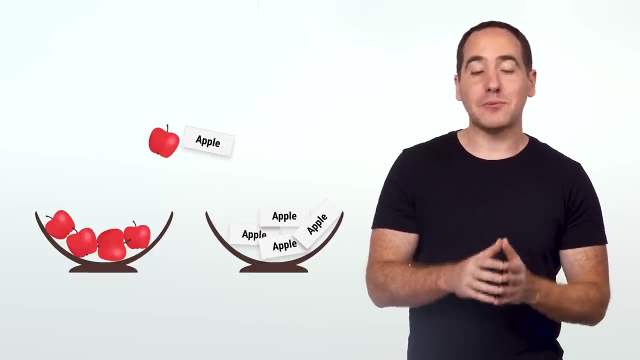 It's basically incorrect if we randomly assign a label from a set to an example in that set. Here's an example to make that clear. Imagine we have two bowls and one contains the examples and the other contains labels. First we'll randomly draw an example from the first bowl, then we'll randomly 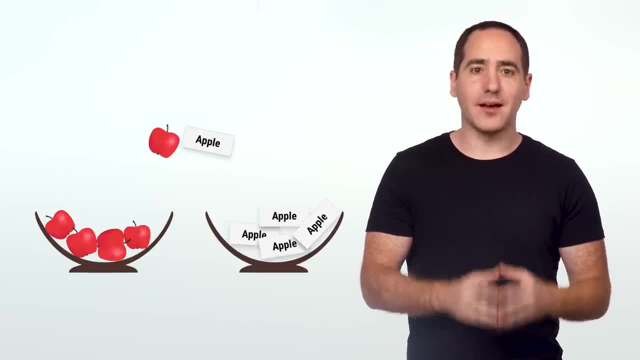 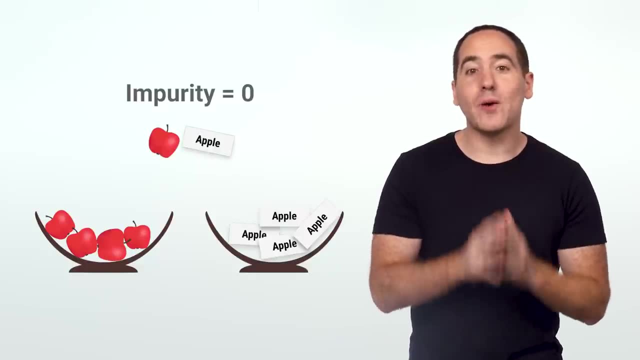 draw a label from the second, and now we'll classify the example as having that label, And Ngini impurity gives us our chance of being incorrect. In this example, we have only apples in each bowl. there's no way to make a mistake. 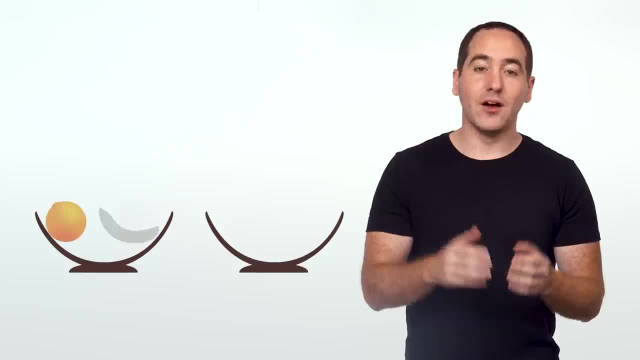 and we'd rather have some empty label. so let's just say the next one, which is a red and vice. so we say the impurity is 0.. On the other hand, given a bowl with 5 different types of fruit in equal proportion, 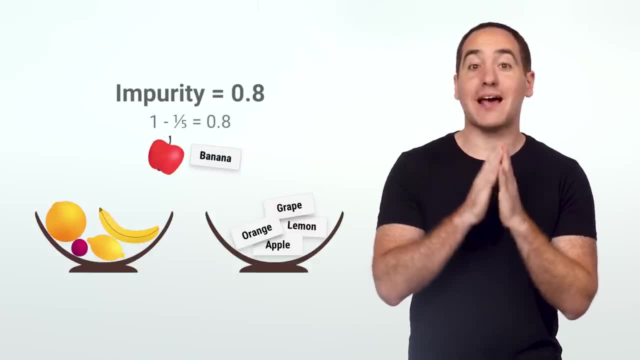 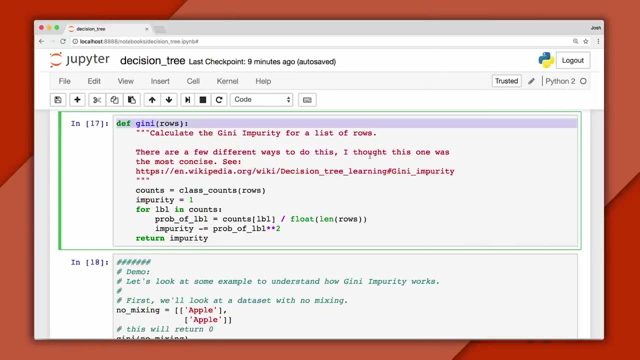 we'd say it has an impurity of 0.8.. That's because we have a 1 out of 5 chance of being right. if we randomly assign a label to an example In code, this method calculates the impurity of a data set. 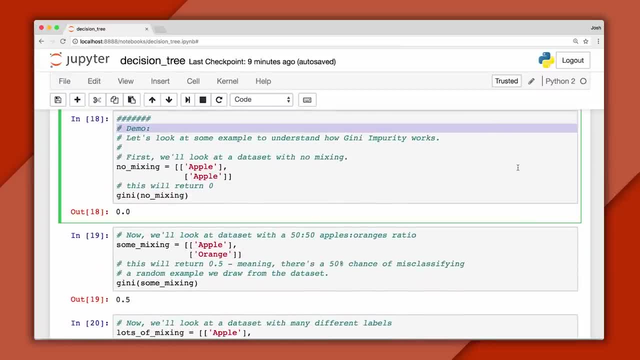 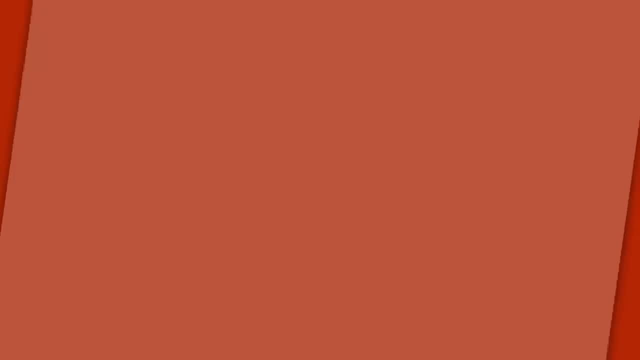 and I've written a couple examples below that demonstrate how it works. You can see the impurity for the first set is 0 because there's no mixing, and here you can see the impurity is 0.8.. Now information gain will. let us find the question that reduces our uncertainty the most. 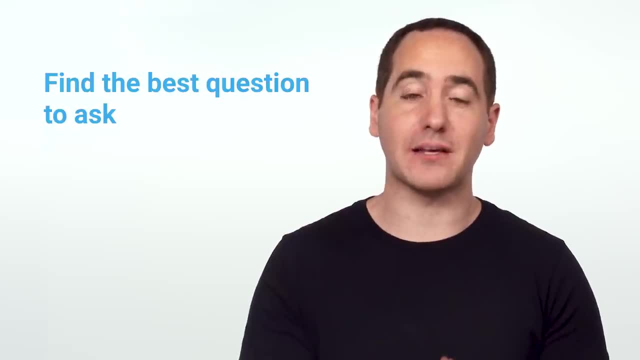 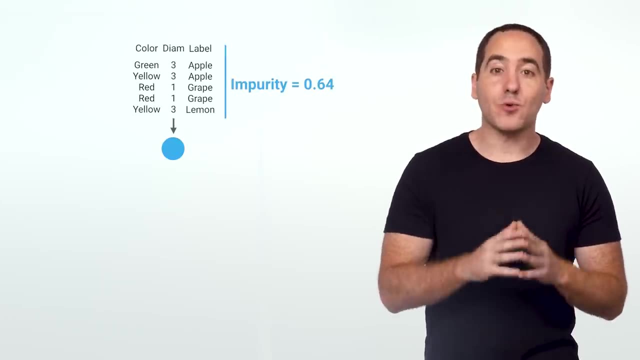 and it's just a number that describes how much a question helps to unmix the labels at a node. Here's the idea. We begin by calculating the uncertainty of our starting set. Then, for each question we can ask, we'll try partitioning the data. 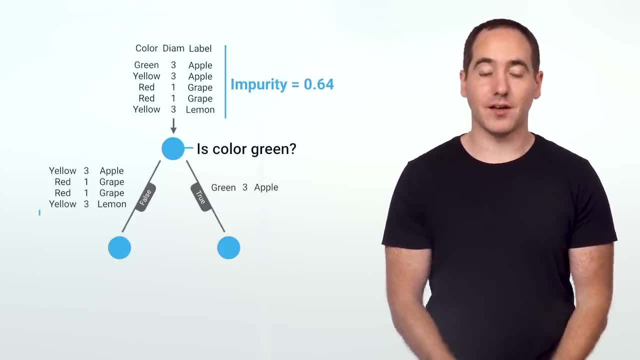 and calculating the uncertainty of the child nodes that result. We'll take a weighted average of their uncertainty, because we care more about a weight of a large set with low uncertainty than a small set with high. Then we'll subtract this from our starting uncertainty. 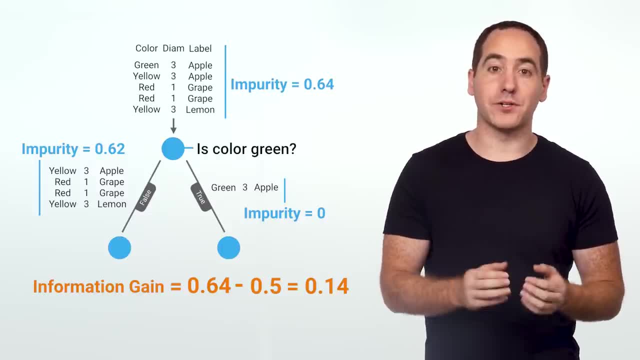 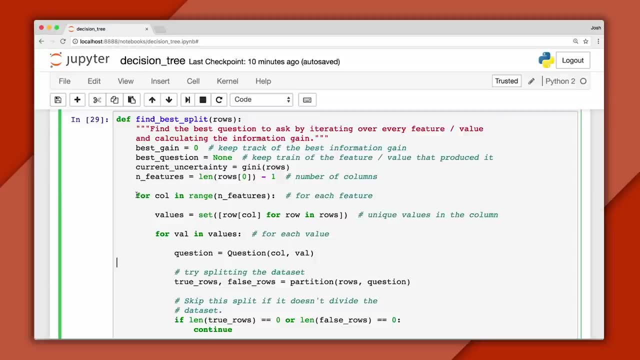 and that's our information gain. As we go, we'll keep track of the question that produces the most gain and that will be the best one to ask at this node. Let's see how this looks in code. Here we'll iterate over every value for the features. 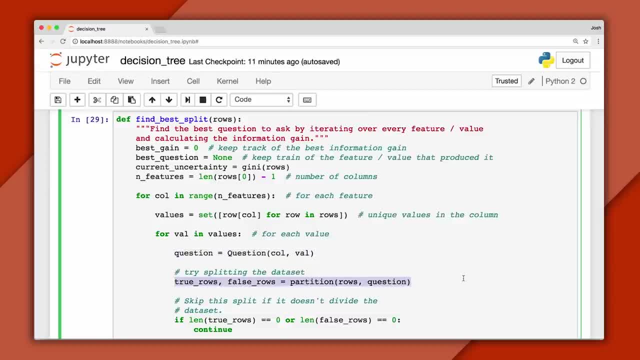 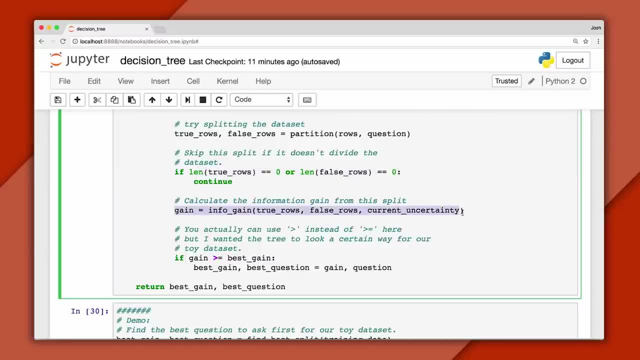 We'll generate a question for that feature, then partition the data on it. Notice we discard any questions that fail to produce a split. Then we'll calculate our information gain and inside this function you can see we take a weighted average and the impurity of each set. 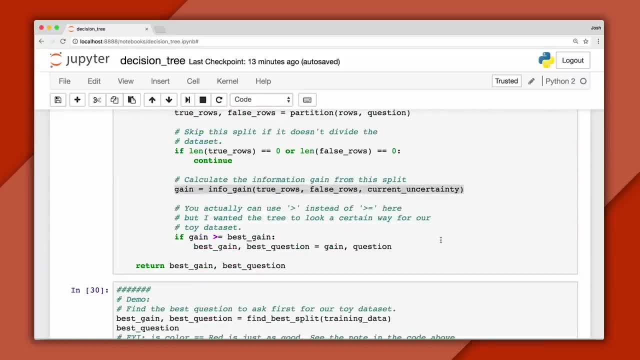 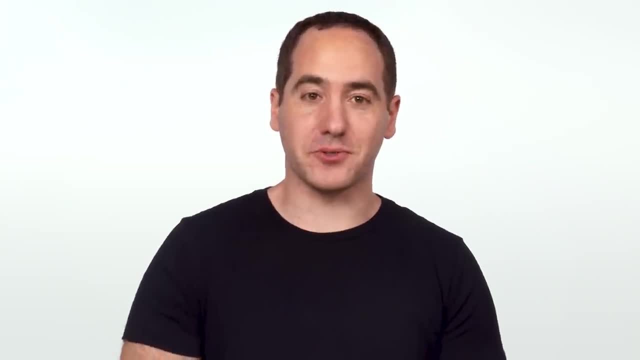 We see how much this reduces the uncertainty from our starting set and we keep track of the best value. I've written a couple demos below as well. Okay, with these concepts in hand, we're ready to build the tree And to put this all together, I think, the most useful thing I can do. 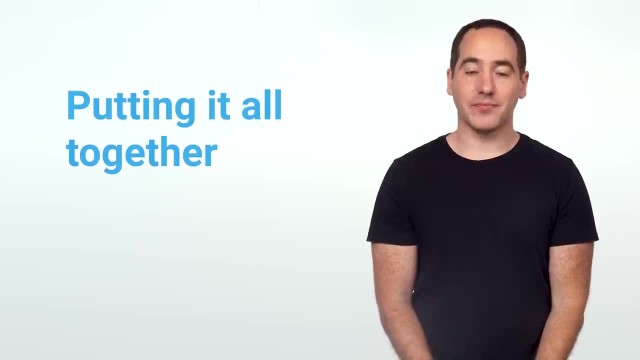 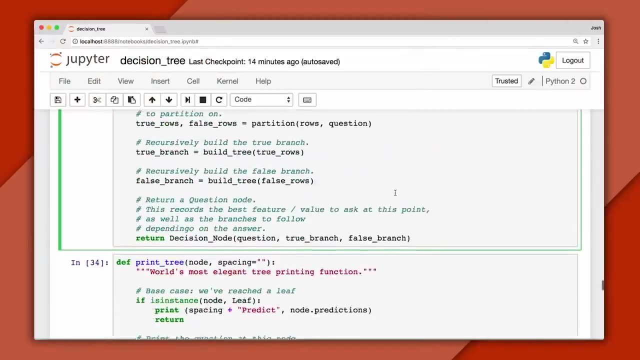 is walk you through the algorithm as it builds a tree for our training data. This uses recursion, so seeing it in action can be helpful. You can find the code for this inside the buildTree function When we call buildTree for the first time. 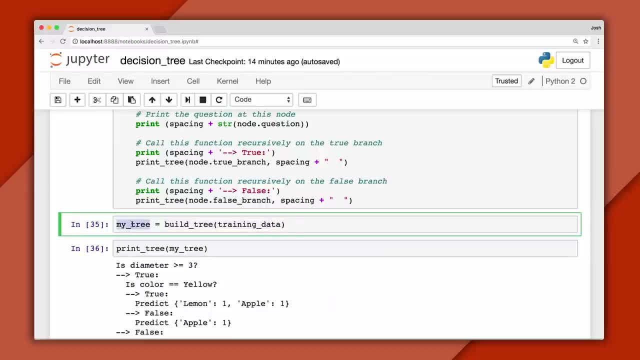 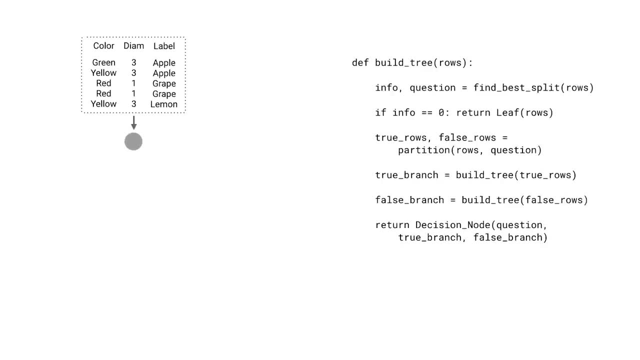 it receives the entire training set as input and as output it will return a reference to the root node of our tree. I'll draw a placeholder for the root here in gray And here are the rows we're considering at this node. and, to start, that's the entire training set. 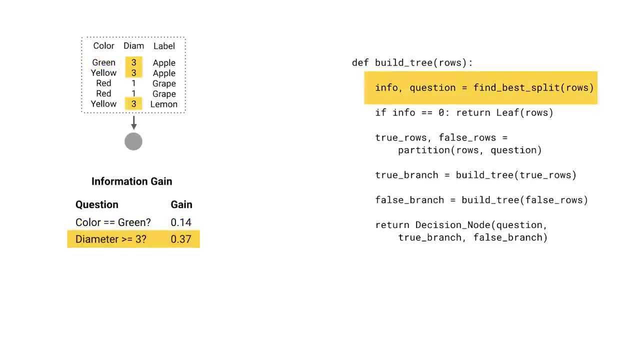 Now we find the best question to ask at this node, and we do that by iterating over each of these values. We'll split the data and calculate the information gain for each one and as we go, we'll keep track of the question that produces. 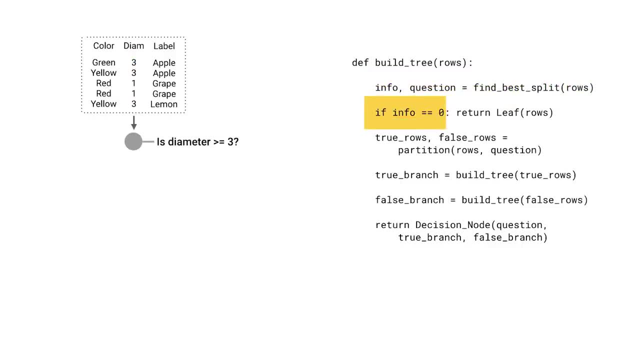 the most gain. Now, in this case, there's a useful question to ask, so the gain will be greater than zero and we'll split the data using that question. And now we'll use recursion by calling buildTree again to add a node for the true branch. 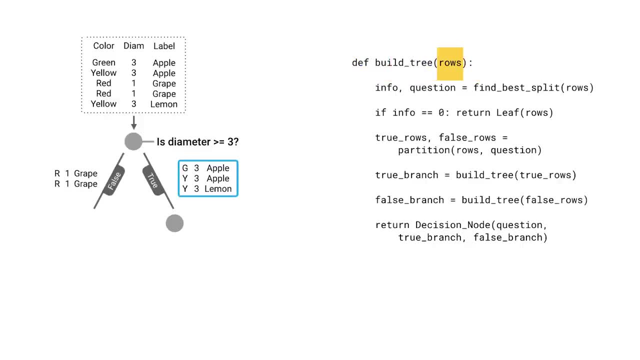 The roads we're considering now are the first half of the split and again we'll find the best question to ask for this data Once more. we split and call the buildTree function to add the child node. Now for this data. there are no further questions to ask. 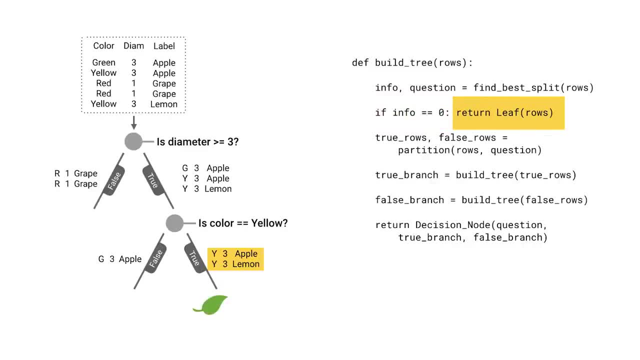 so the information gain will be zero and this node becomes a leaf. It will predict that an example is either an apple or a lemon, with 50% confidence, because that's the ratio of the labels in the data. Now we'll continue by building the false branch.